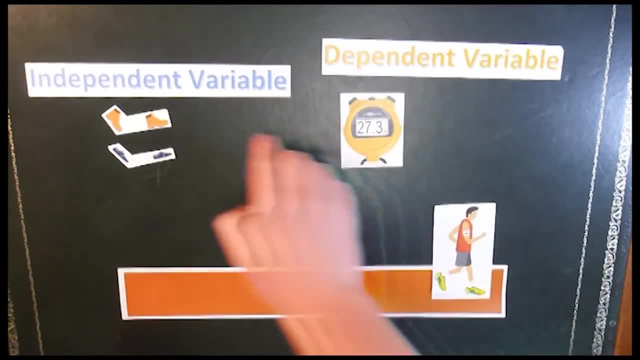 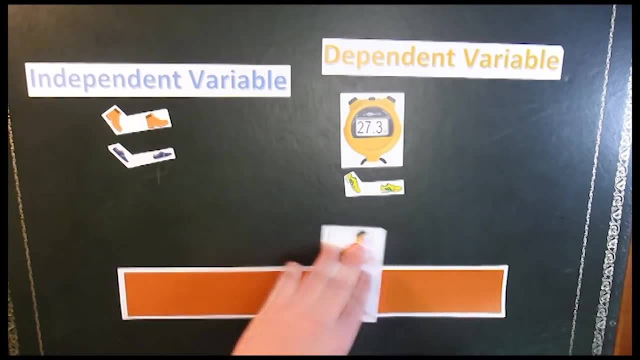 dependent variable. It depends on our independent variable. You've got a time of 27.3 seconds with his runners. We reset him back to the start, We put his casual shoes on, We start the timer. He runs the hundred meters and this time he got a time of 30.2 seconds. So a little bit. 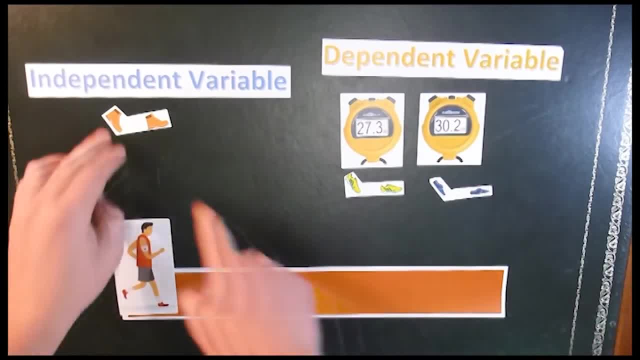 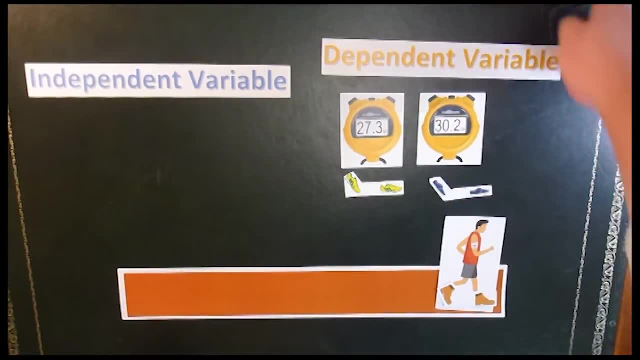 slower. this time. We take him back to the start, We put his boots on, We start the timer. He runs the hundred meters. We stop the timer and this time he got a time of 33.3 seconds, which was his slowest time, So we can say that he runs. 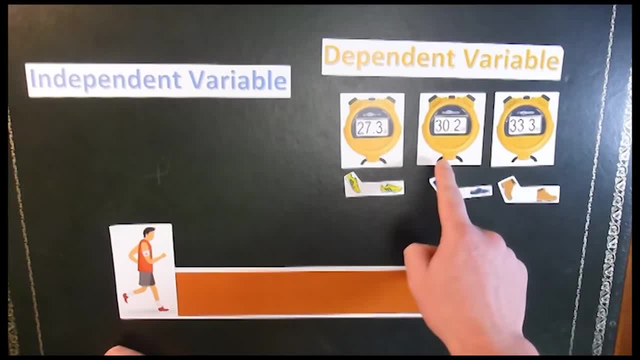 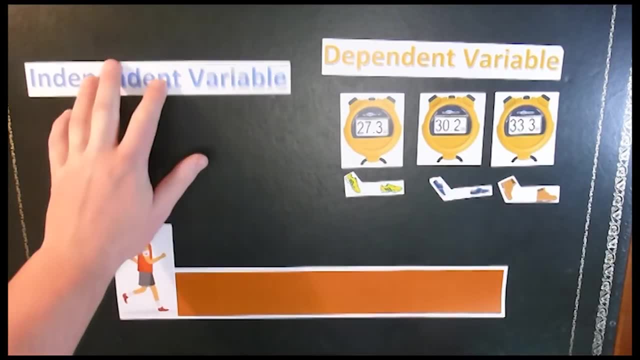 the fastest with his runners, followed by his casual shoes, and then he runs the slowest in his boots. But that's not everything to this experiment. There's a few other things that we need to consider. The first thing to consider is the weather. We need to make sure that the weather was kept the same each time. 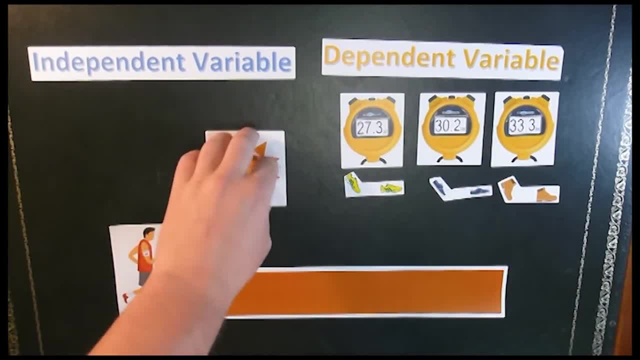 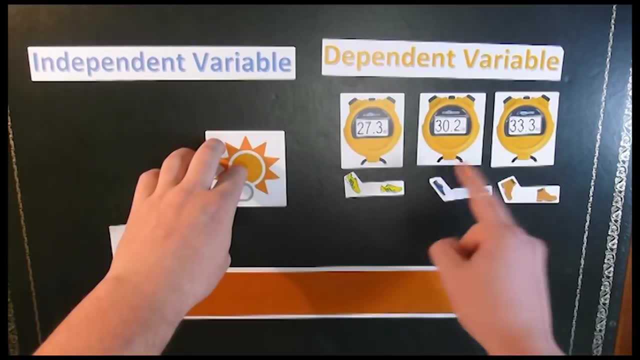 he ran the hundred meters If it was sunny when he was wearing his runners, but if it was raining when he wore the other shoes, that's not really a fair comparison, because the weather could have had an impact on his ability to run. The clothing that he was wearing is also 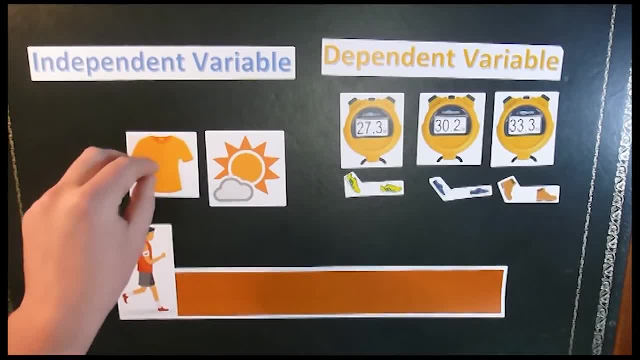 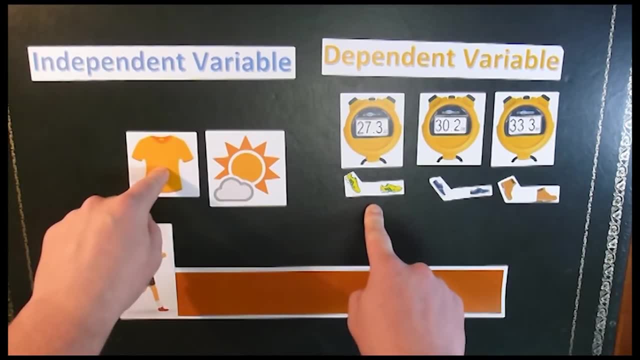 something that we need to consider. We need to make sure that he was wearing the same clothes every time he ran this hundred meters. If he was wearing running gear, wearing his runners, he had to be wearing running gear for the other ones as well. Otherwise, his clothing could have. 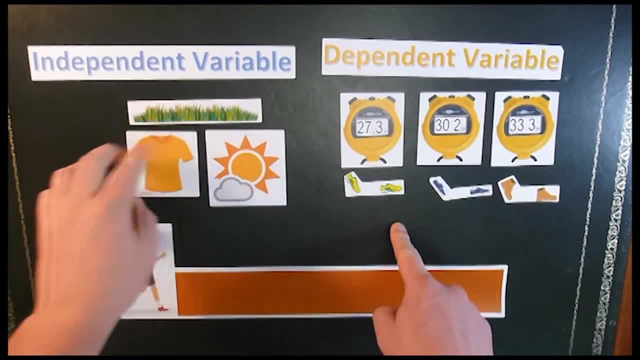 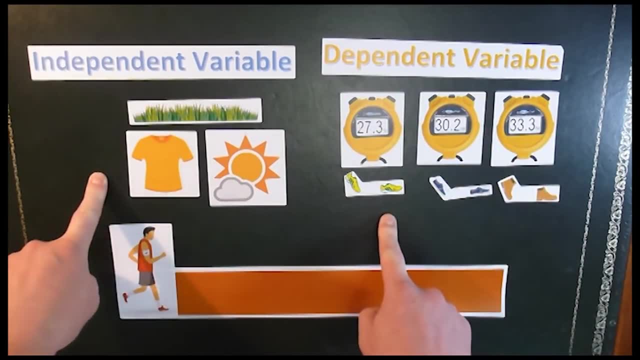 affected his time Same with the surface If he was running on concrete or wood or grass. we need to make sure that that was the same every time he ran this hundred meters, so that any difference in time was mainly just due to the shoes. 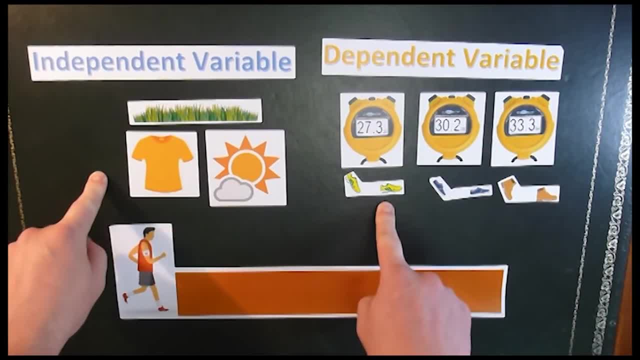 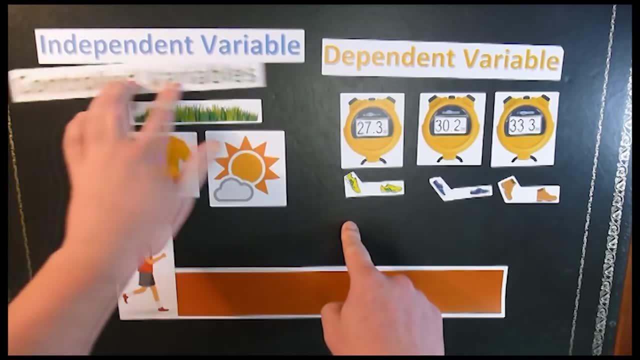 that he was wearing. That's what we're trying to achieve: an accurate and fair comparison between the types of shoes, Because these are the things that we're trying to control in this experiment. we call them controlled variables, And that's it for today's lesson. I hope you learnt something. Please like and. 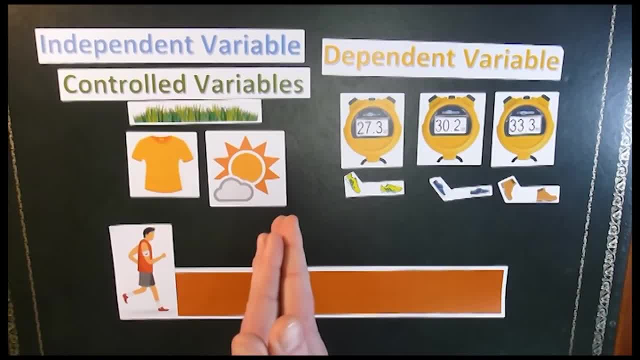 subscribe if you want to see more of these videos, and I will see you next time.